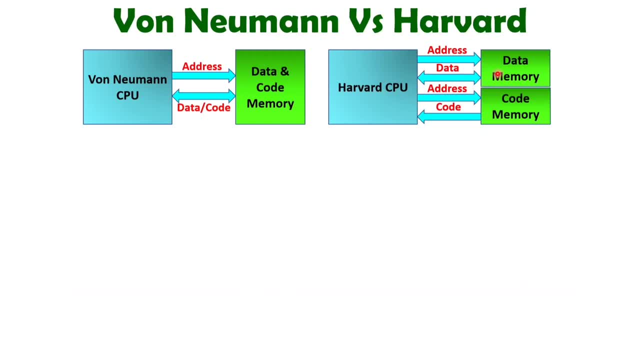 in Howard CPU you will be observing, data memory and code memory are different. So here system bus that is also separate for data and code. Here you can observe, in terms of interfacing complexity is less with Von Neumann CPU. With Howard CPU complexity is more in terms of interfacing. 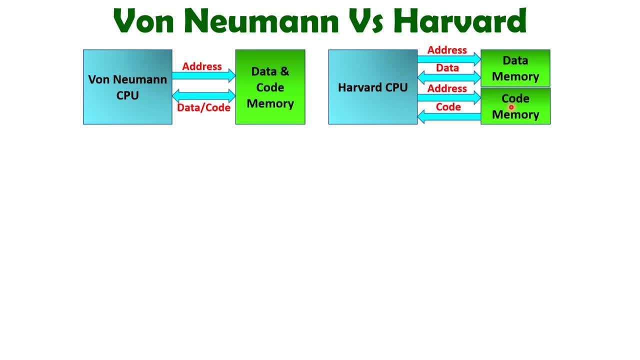 Why The reason is: separate memories are over here, But here, my dear students, when you execute any program, at that time data and code both cannot be accessed simultaneously in Von Neumann CPU. So you can say: Von Neumann CPU are slow. Why The reason is? 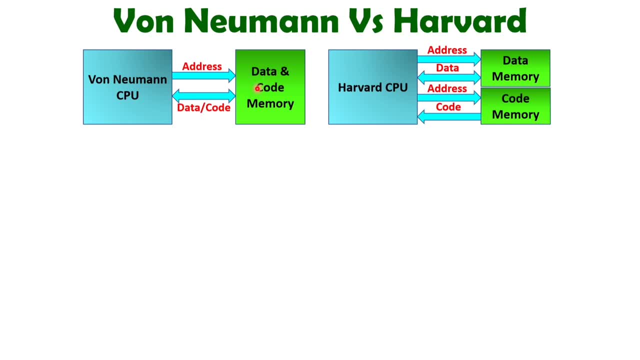 separate machine cycles are required for data access and code access, While with Howard architecture data memory and code memory that is separate, So simultaneous access of data and code is possible As well as here, interfacing. complexity is more. There are a few more basic things that you should. 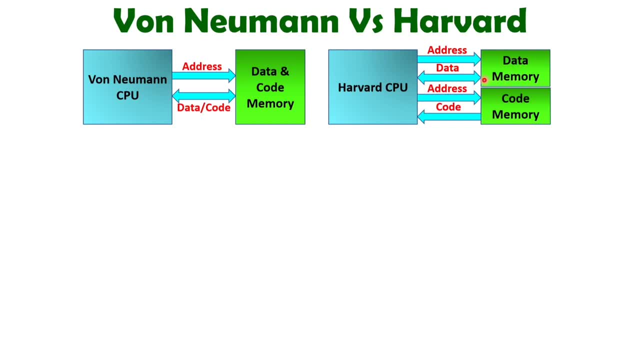 know like data memory that could be read by CPU or write by CPU. That's why it should be RAM. You can see here bidirectional data is shown. So data memory must be RAM, But with code memory CPU will read data of code memory, right? So you will be observing that is unidirectional over here. 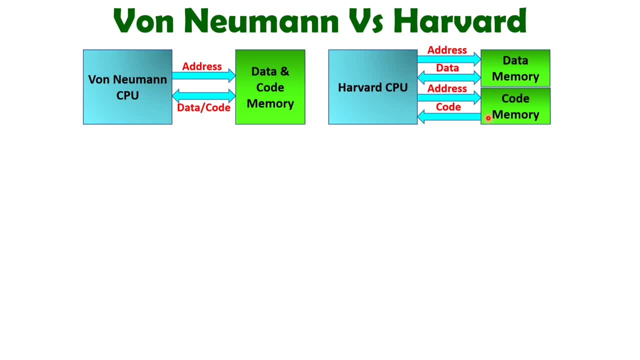 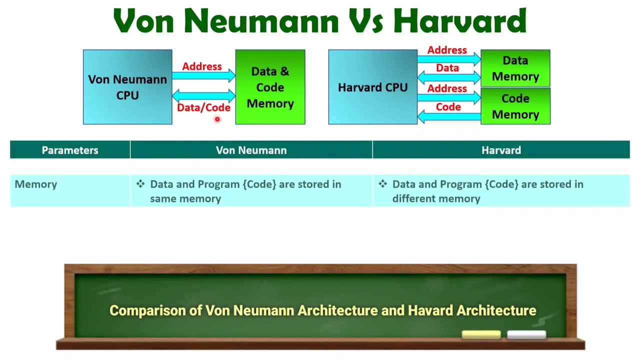 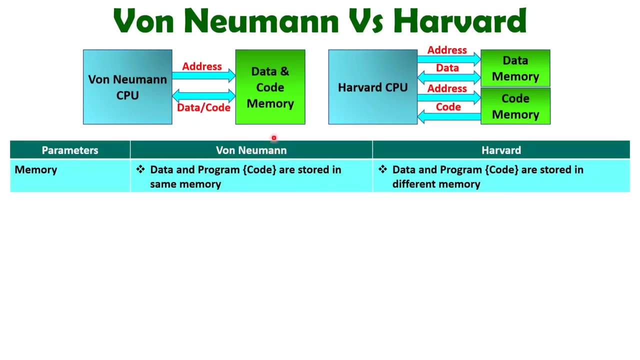 That is ROM only, as we are just reading code over here with Howard CPU. Now I'm going to explain you the comparison with respect to various parameters. So when it comes to memory, you should know Von Neumann architecture, that is, having common memory over here, right Data and code? Code means 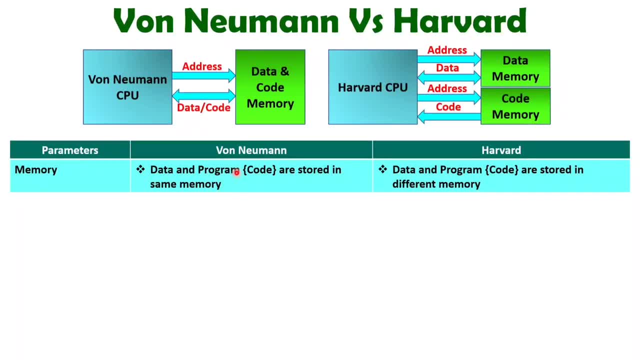 program, You can say instruction as well, right, So that is stored in a same memory with Howard structure Data and program. that is there with separate memories. Here when we talk about memory type, then you should know here this common memory that should be RAM only. Why The reason is this code that we will. 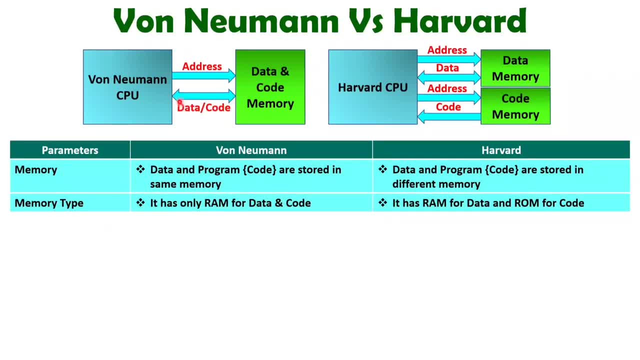 be reading only, But in data you may perform read and write operation. So this should be bidirectional, right. Bidirectional means it will be RAM. In RAM you can read as well as write the data. So you'll be observing, with Von Neumann CPU, this main memory, that will be RAM only. But with Howard CPU you will. 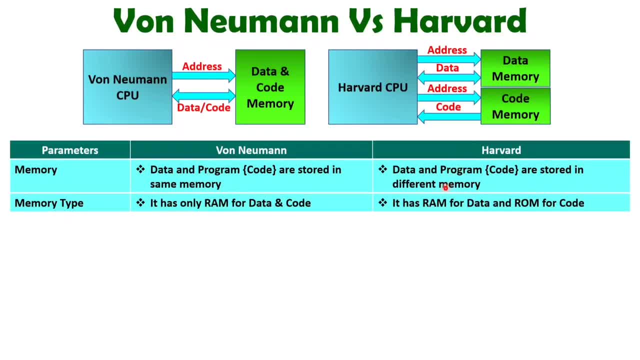 be having two separate memories: Data memory that is there with RAM and code memory that is there with ROM. Why? The reason is: with data we will be performing read as well as write operation, right? So data will be bidirectional over here. So that should be random access memory with data. 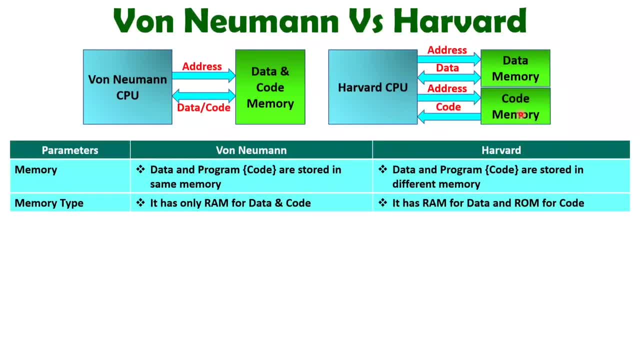 And with code you will be just reading and writing data. So that is the reason. So data will be reading data, right, It should be non-volatile. You cannot change the code, So code should be stored with ROM memory only. So here with Howard architecture, two separate memories are there. 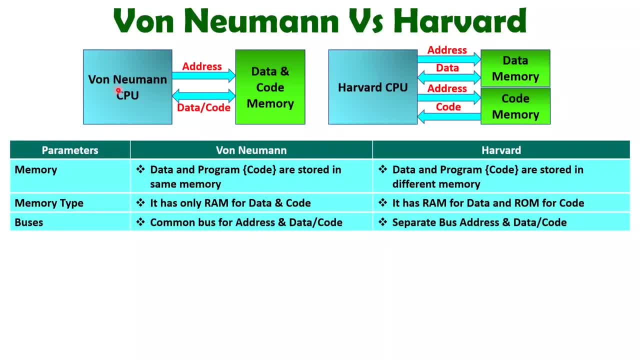 Here. when it comes to buses, then with Von Neumann structure, as we have common memory, common system bus is there. System bus means it includes address data as well as control signals, But with Howard architecture, separate buses will be there. Why The reason is? 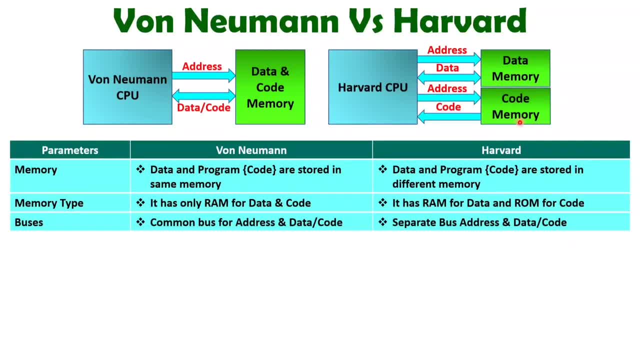 here separate signaling will happen with data and code memory, as both are separate. So here you will be observing: control signals are more over here compared to this Von Neumann structure. So in terms of bus interface, Howard CPU is complex compared to Von Neumann CPU. 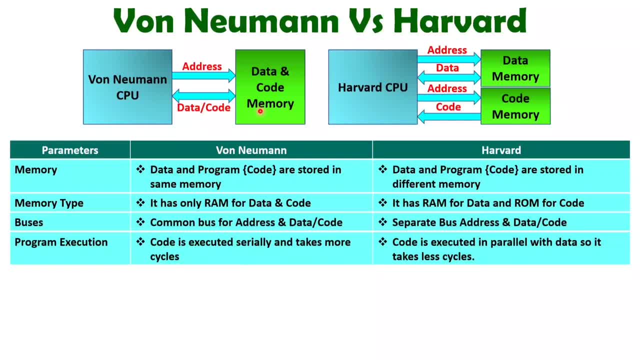 Here when it comes to program execution, then you should know here this code execution that will happen serially One by one. instruction will come over here inside CPU and it will execute instructions one by one serially. Here when it comes to access data, then code and data access, that cannot happen. 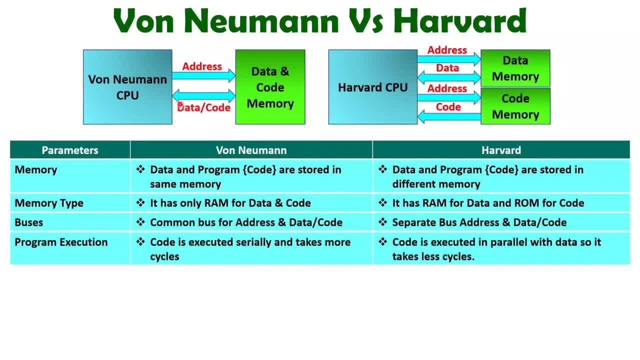 simultaneously, So serially. code execution will happen along with that. CPU will use data, But both of these things are not happening simultaneously. It will happen serially, But when it comes to Howard architecture you will be observing, execution of instruction will happen in sequence only, But along with instruction. 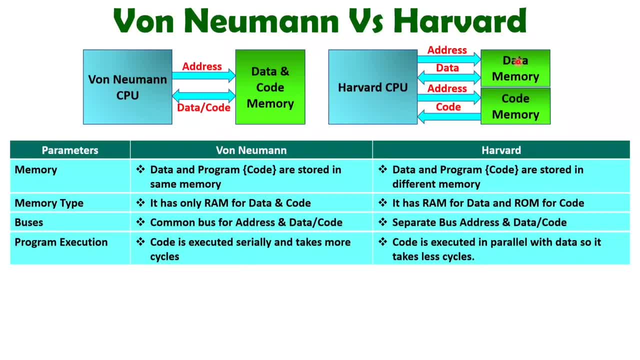 as if CPU wants to access data memory, then that is possible in parallel, right? So read and write data is possible in parallel with code execution. So Howard CPU- that is faster. Why? The reason is Howard CPU will take less number of cycles as you have separate data and code memory. 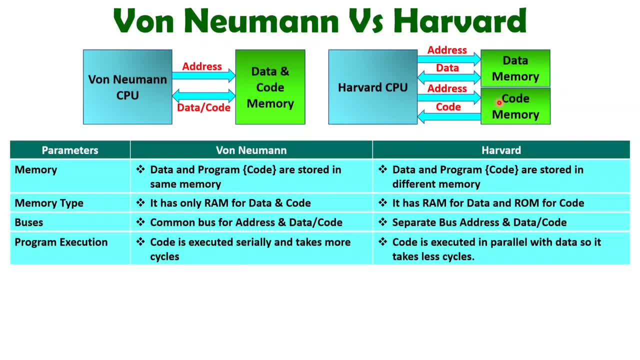 Simultaneous operation of code and data is possible. It will take less machine cycles to execute program. right, But with Von Neumann complexity is less, but it is slower Here when it comes to code and data transfer. then you can say that data or code that is. 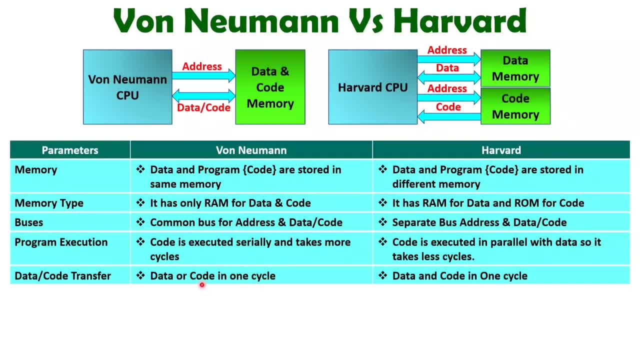 getting executed in a single cycle. Both cannot get executed in a single cycle at the same time. Either you execute data or you execute code in a one cycle. But with Howard CPU, data and code- both can get executed at the same time in a single cycle. So that is. 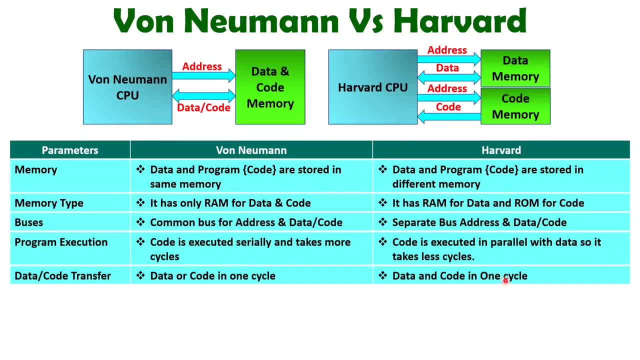 how Howard CPU is having advantage. But disadvantage is what you need: to have many control signals over here, compared to Von Neumann structure. When it comes to control signals, as I have told you here, only one memory is there, so less control signals are required, But with two separate memories you need. 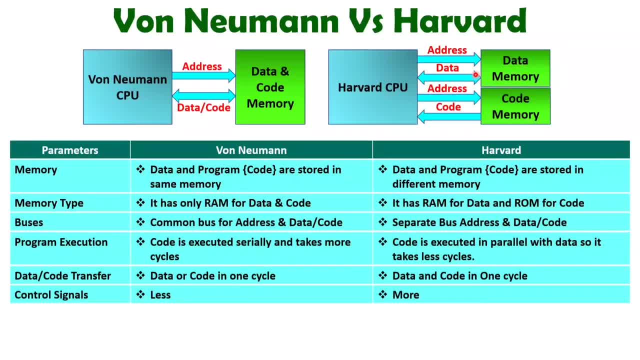 extra control, Like you see here, with data memory memory read and memory write control signals that we need to provide. with code memory, We need to provide memory read control signal right, While with this Von Neumann structure you just need to have read and write control signals with this memory right. here See separate memories are there, So memory. 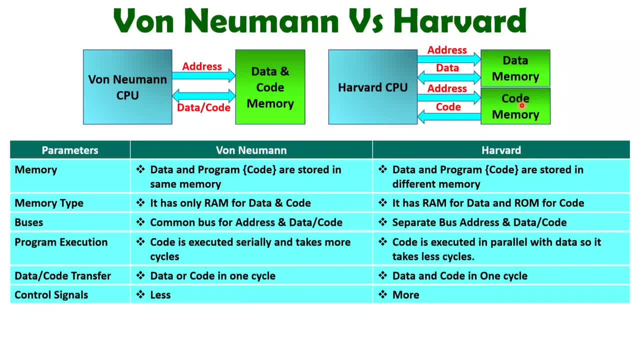 selection. that is also an essential thing that we need to have. So all those things that comes under control, control signals, so you can say that one human is having less control signals compared to howard architecture in terms of space, you can say, with one human structure, you need less space. why? 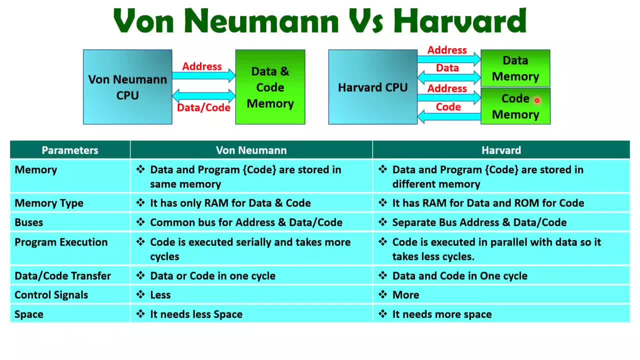 the reason is: common memory is there, but with howard cpu you need to have more space. why the reason is here? two memories are there, but along with that interfacing bus, that is also increasing. that's why you need to have more space. see, it is not only about memory which acquires space.